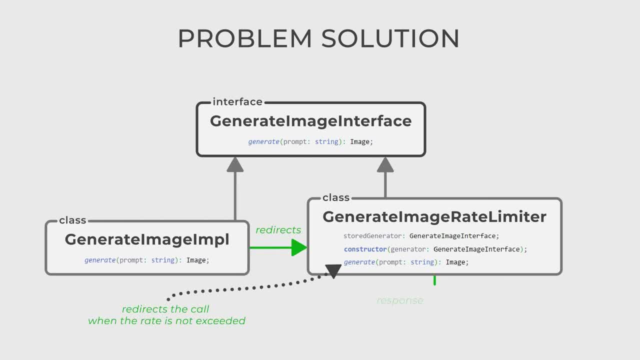 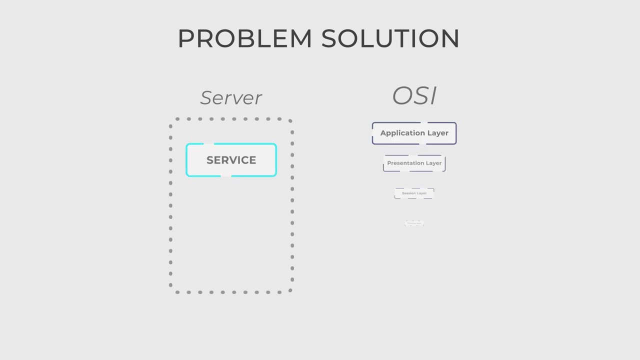 to redirect the call when the rate is not exceeded. Otherwise, when the rate is exceeded, this class becomes a lightweight shield that will prevent the heavy work from starting and will immediately return an error to the client asking to repeat the same request after a delay. In practice, you don't need to create a unique. 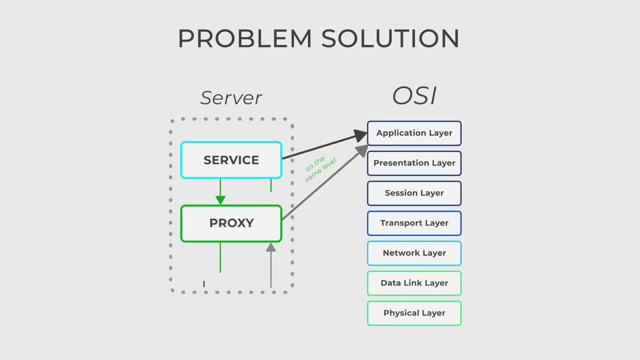 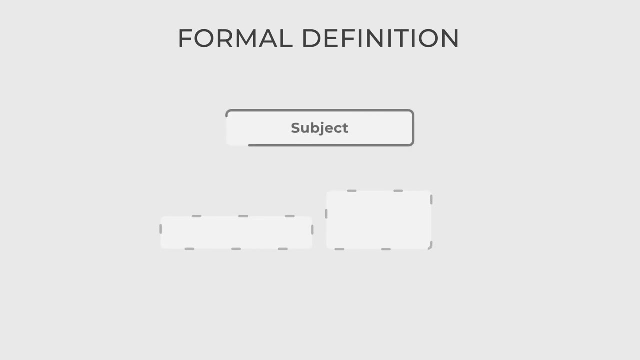 rate-limiting proxy for each specific class, There is a general solution that can also be in a different network layer, so your server will not be overloaded due to requests that should be rejected immediately. There are three actors in this design pattern. The first subject is a generic 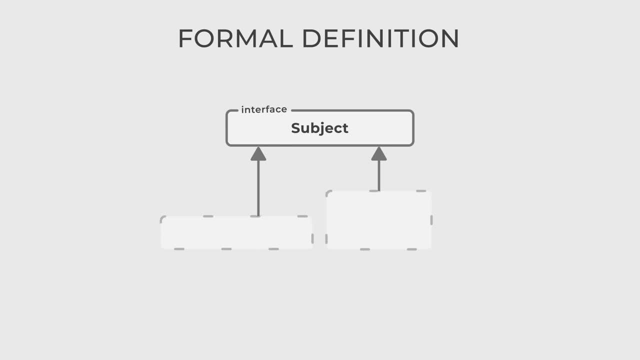 proxy and the second subject is a real object. The real subject and the proxy implement. This allows you to use a proxy instead of a real object. RealSubject is a class that represents the real object or service that the proxy controls access to And, of course, Proxy. 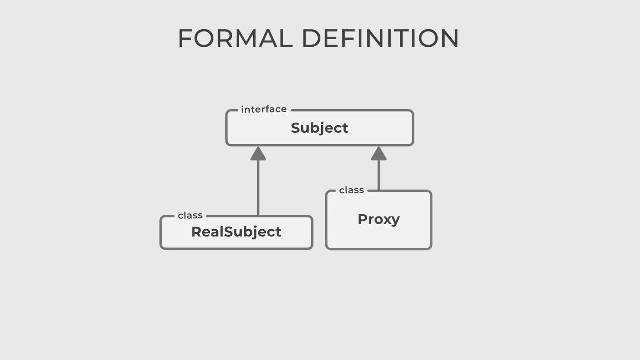 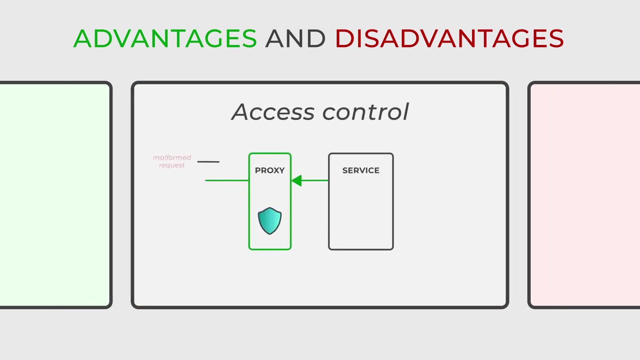 a class that implements the same interface as the subject. It contains a reference to the real subject and controls access to it, adding any necessary functionality. In terms of benefits, the proxy pattern enhances access control By enabling you to manage the permissions and access to the real subject, adding an extra layer of security. 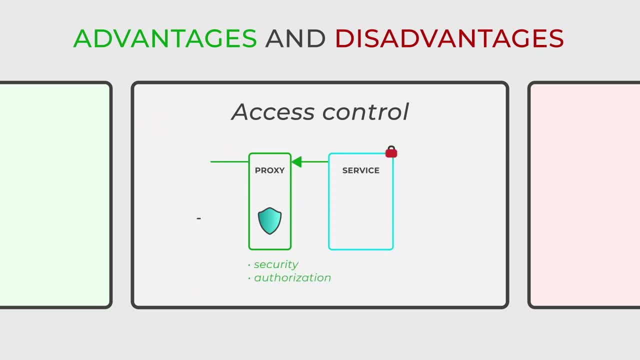 or authorization. This can be particularly crucial in scenarios where sensitive information or operations are involved. Additionally, it aids in efficient resource management, as proxies have the ability to handle resources related to the real subject. This contains lazy initialization, caching and releasing resources when they are no longer necessary, contributing to a more 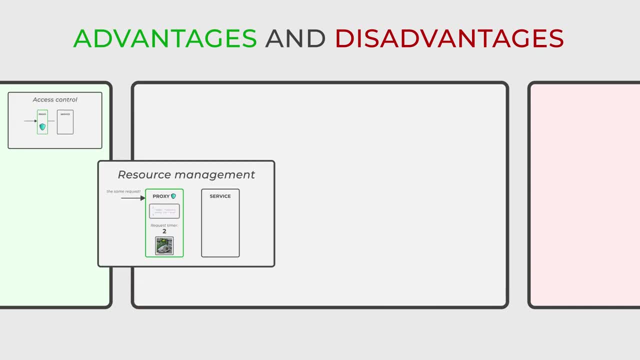 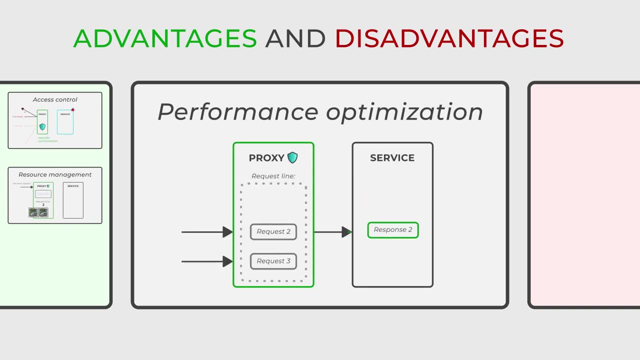 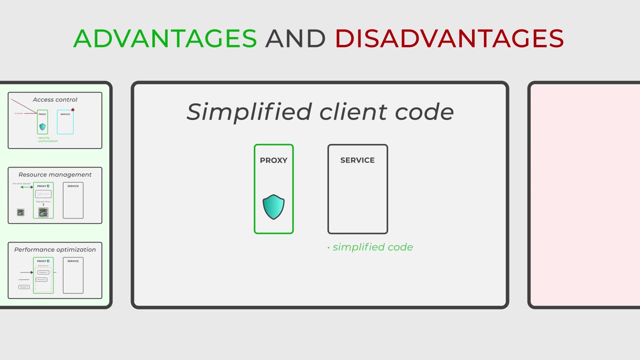 optimized use of system resources. Furthermore, Proxy can optimize the performance of the system. For example, it can postpone the creation or execution of resource-heavy objects or tasks, or reuse just calculated results. Lastly, the client code becomes simpler and more straightforward. when using the. 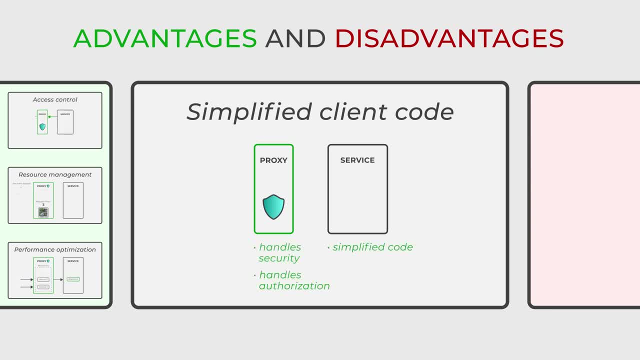 proxy pattern. The complexity of functionalities or interactions is encapsulated within the proxy, making it easier for the client code to interact with the real subject. On the other hand, there are some disadvantages to consider. The introduction of the proxy pattern can lead to.